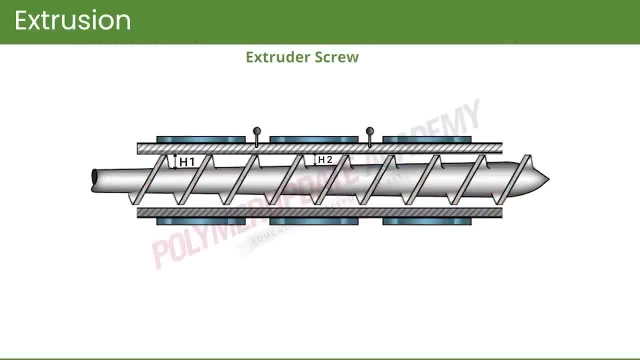 feed zone. The depth of the screw goes on decreasing along the length of the screw. The depth is more in the feed section as compared to that in the compression zone. When the depth decreases, it reduces the volume and increases the melt pressure. The ratio of depth 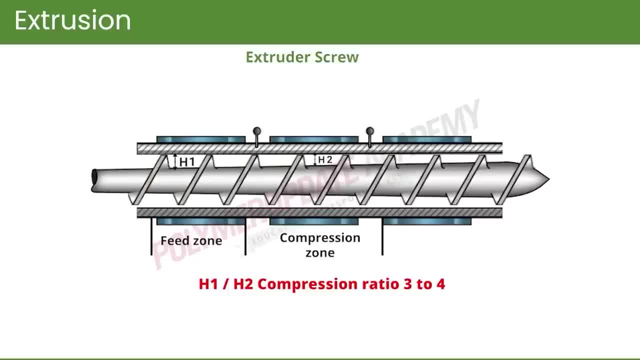 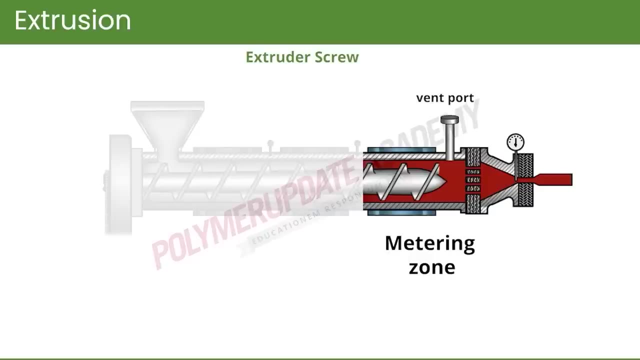 in the feed section to that in the compression zone is called the compression ratio. Most commonly used compression ratio is 3 to 4.. Compression zone is also known as plasticizing zone. In metering zone the melt is conveyed and the vent port optionally provided allows the removal of solvent. 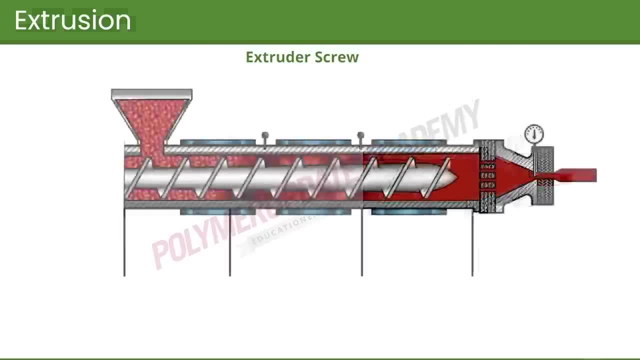 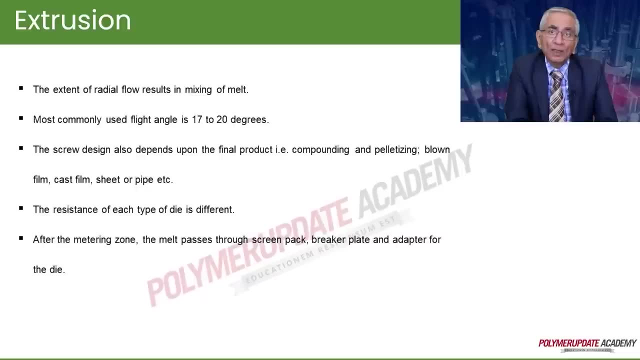 or monomer vapors or any air that may be trapped. The length of feed zone, melting or plasticizing zone and the metering zone are designed differently for different reasons. The extent of radial flow results in mixing of melt. Most commonly used flight angle is about: 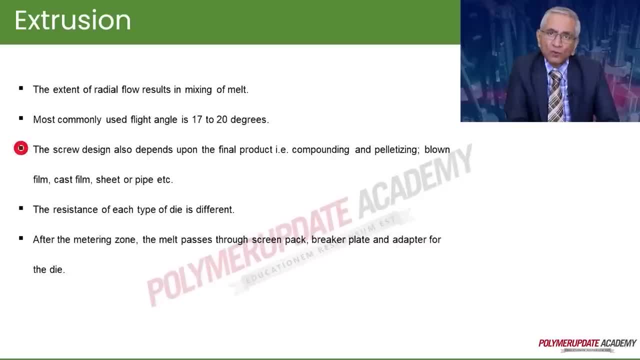 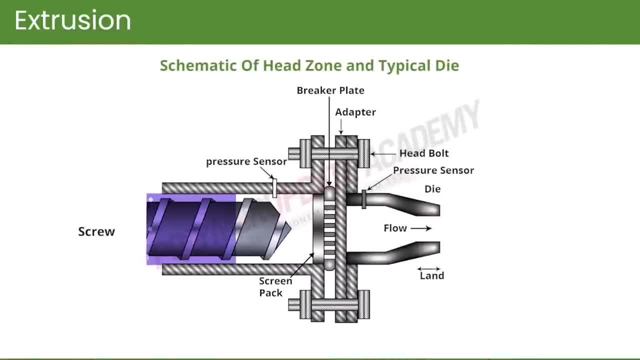 We can see the action of the die. We can see the action of screen pack and breaker plate. The screen pack, as I said earlier, arrests any agglomerates or non molten past. Every single agglomerate will not be able to pass through the screen pack because these are small screens. The large 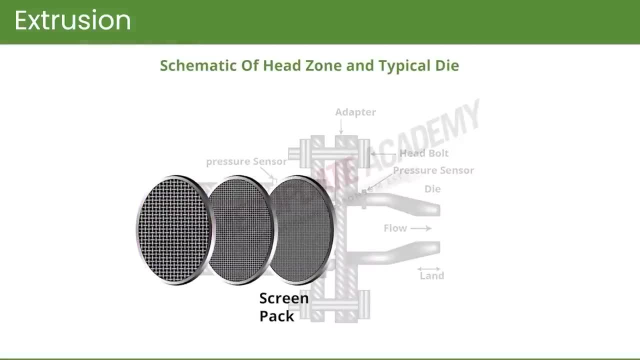 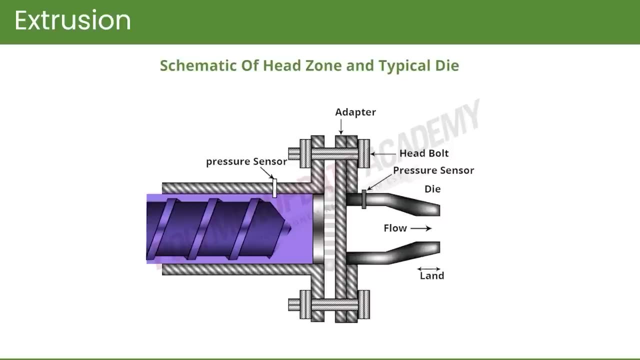 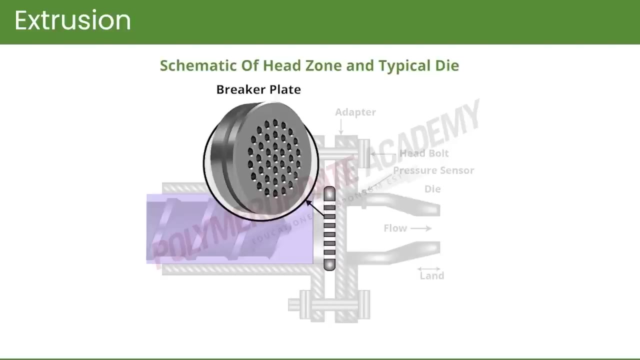 side screen is first placed, then smaller size, then smaller size. Thus the total pressure drop for the liquid to flow through the screen pack is reduced or minimized. The breakers plates have many orifice of larger size, much larger size than that compared to the screen pack and these 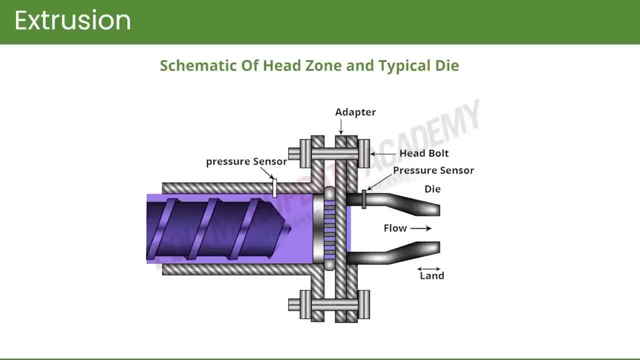 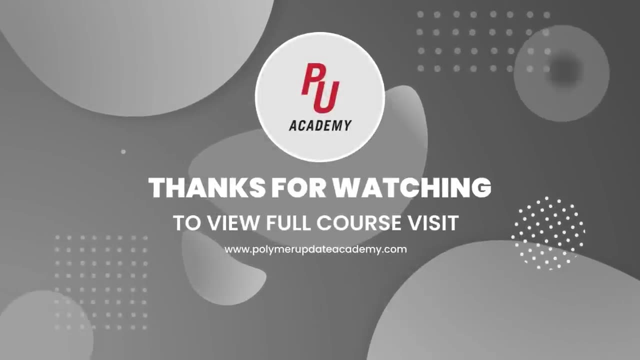 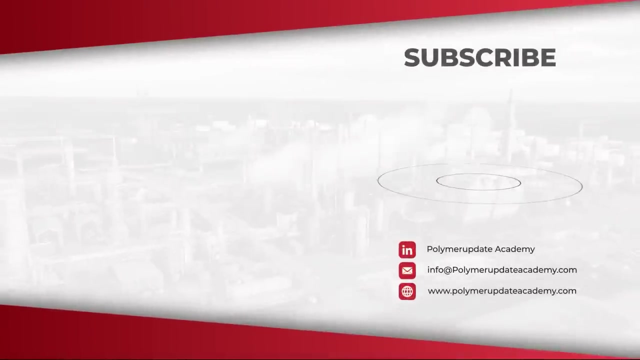 holes allow the material to flow smoothly and any radial component of the flow is stopped and entire flow starts moving in the axial direction, as it is shown over here in the die.